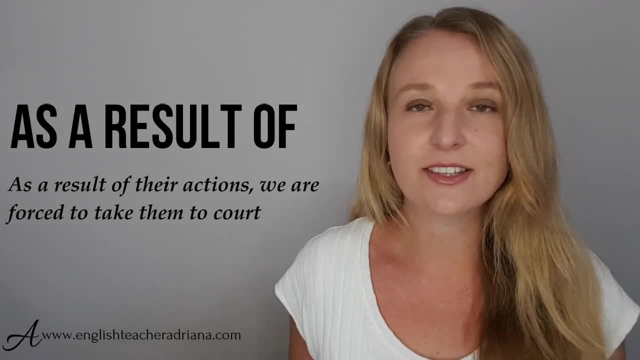 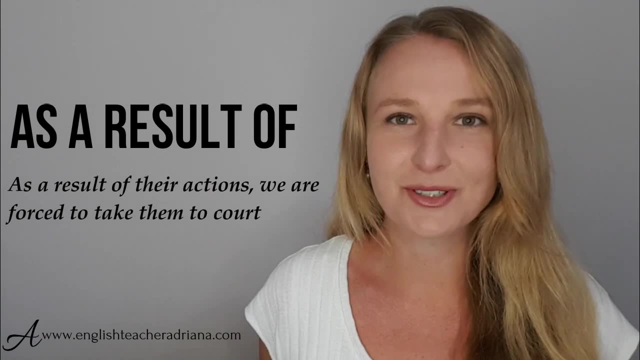 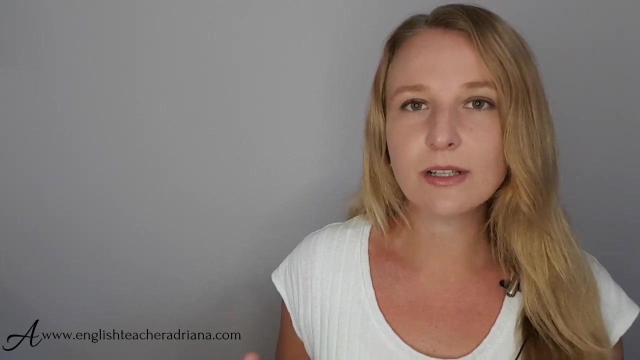 so here, instead of saying because of, we are using as a result of. it's a great synonym to be using examples like this careful pronunciation: as a result of, as a result of, but if you need to be a little bit more informal, so express that something will happen, something will occur. 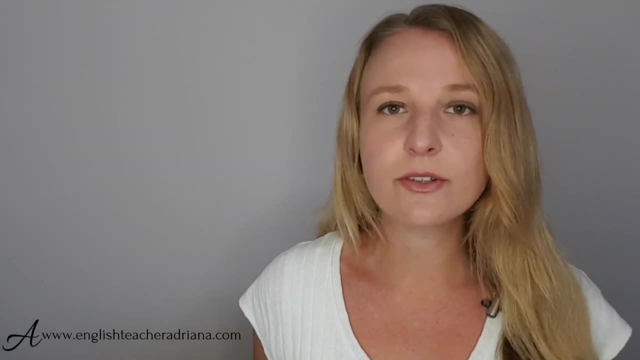 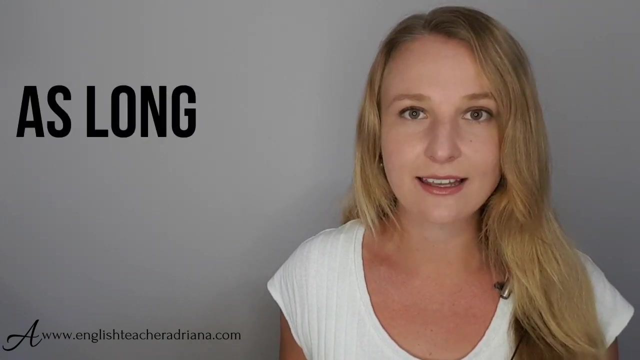 provided. something else has happened, for example, in the sentence because you're going to the shops, can you buy me some milk? now, here, instead of using the word because we could use the phrase as long as. as long as you're going to the shops, could you please buy me some milk? so here we're talking. 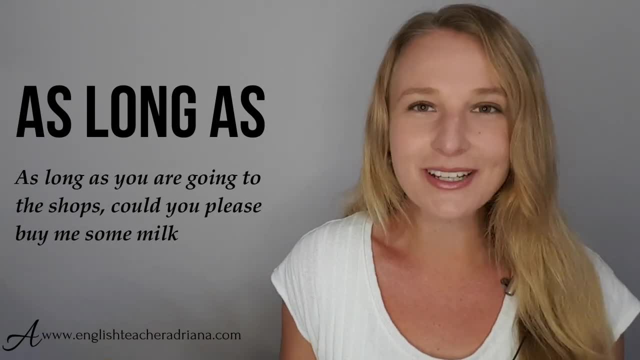 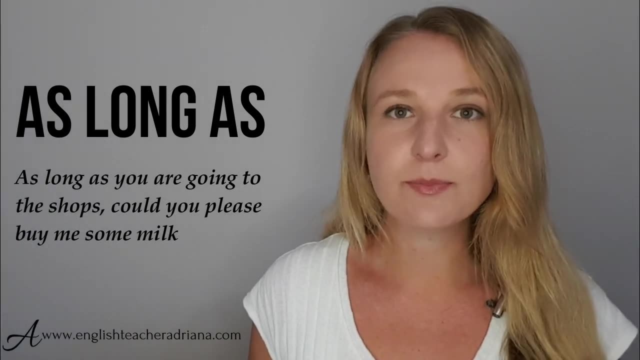 about the fact that you're going to the shop and the result because you're going there. so, as long as you're going to the shops, could you buy me some milk? please note, guys, that this is very informal, great to be using with friends, family, people that you have a good relationship with, and 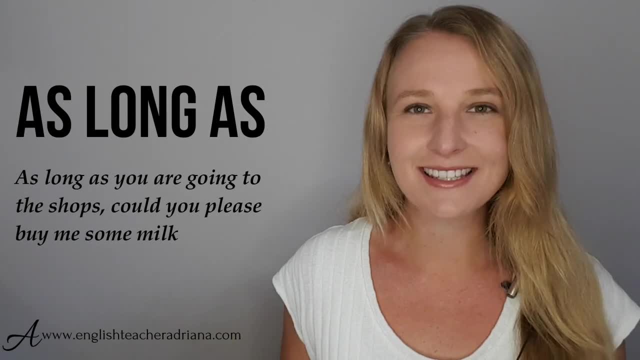 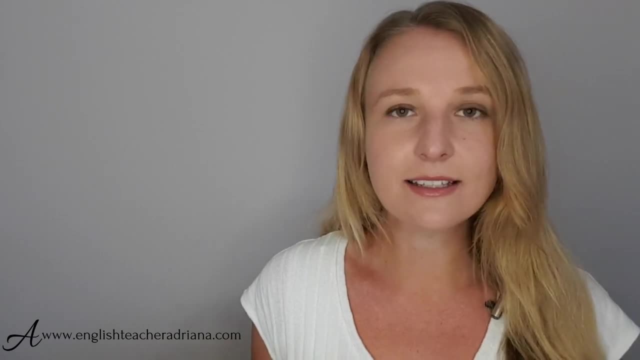 you would be honest and honest with what you say when you're using it. to put it in the context of: it is often used in conversational settings: Careful pronunciation: as long as, as long as, But a more formal phrase you could use instead of as long as is the phrase being, as being, as. 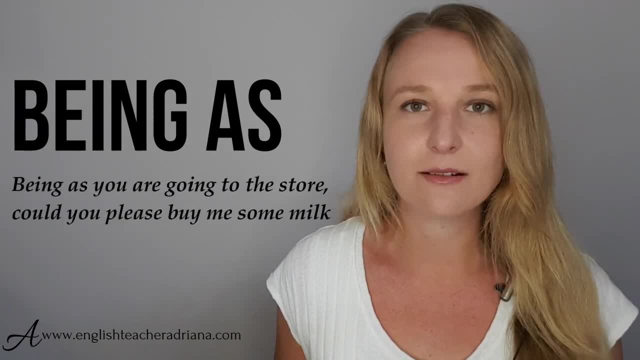 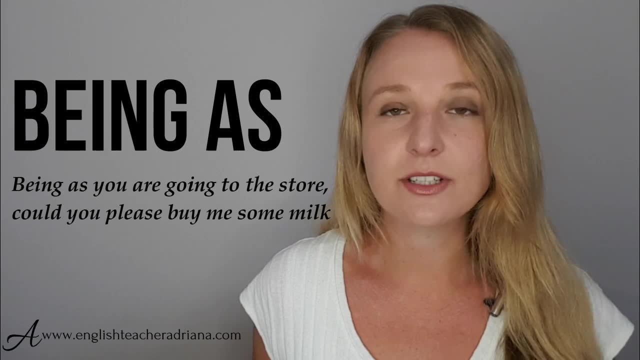 For example, being as you're going to the store, could you please buy me some milk? So this is great to be using with people that you don't have a good relationship with. It is very formal. I don't use it quite often, but many English speakers do in formal settings and it's a great phrase to 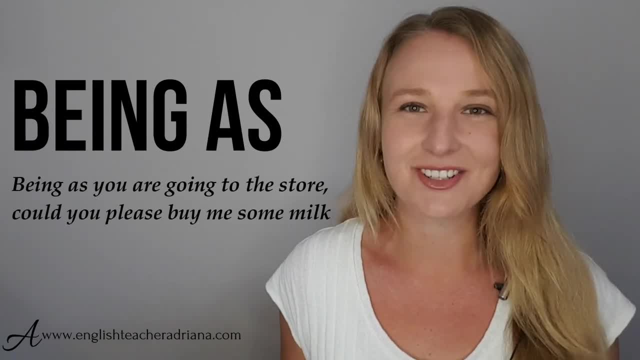 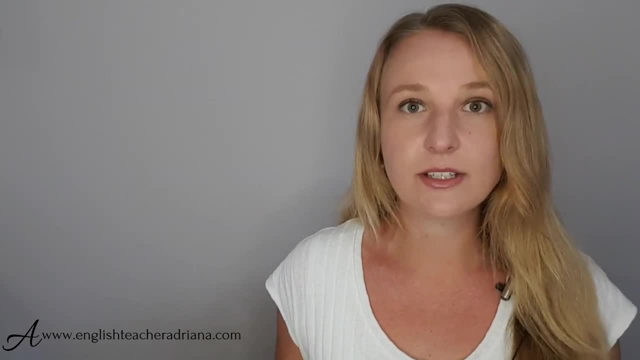 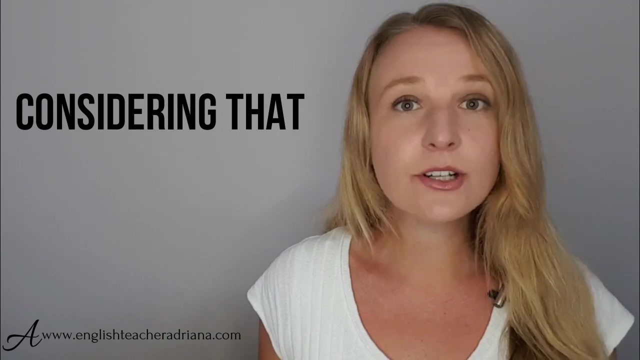 be using in a work setting with people that you don't have a good relationship with. Careful pronunciation being as being as, But a phrase that I do use quite often and also has a similar meaning to as long as and being as, is considering that, For example, considering that you're going. 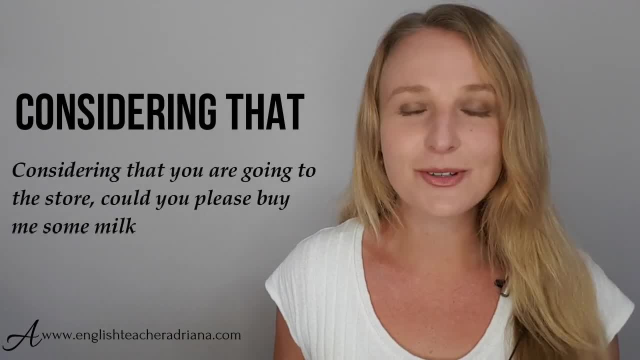 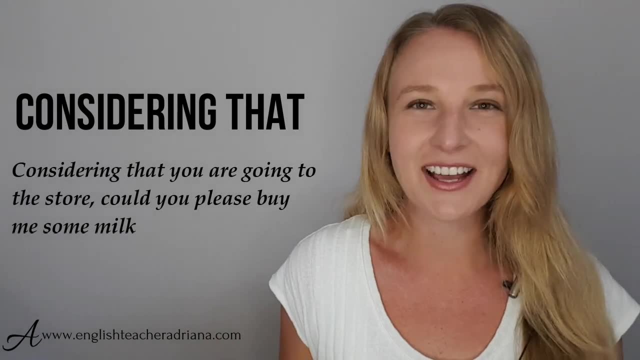 to the shops. could you please buy me some milk? You'll hear this phrase being used in a lot of TV shows and movies. It's used a lot in everyday conversational English, So if you would like to ask somebody to do something, you can use it, But if you don't have a good relationship with people, 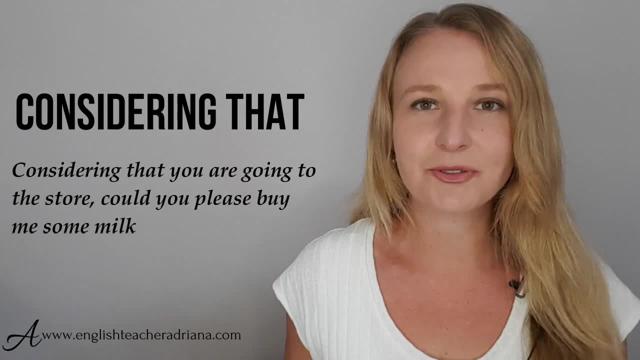 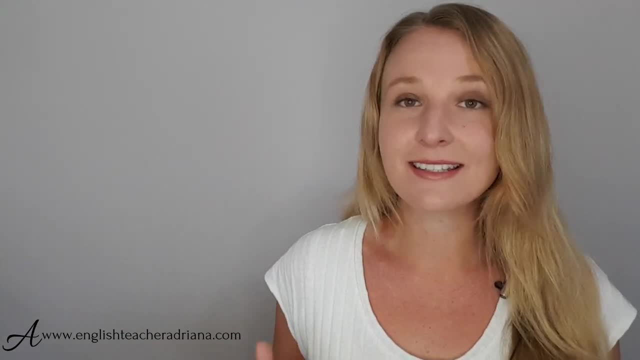 that you're seeing something because they're going somewhere. considering that is a great phrase, to use Careful pronunciation. considering that, considering that- Also very similar phrase to considering that- has the same meaning as a phrase. seeing that, seeing that, For example, seeing that. 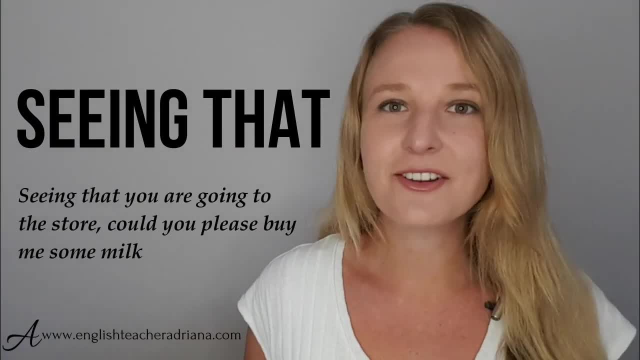 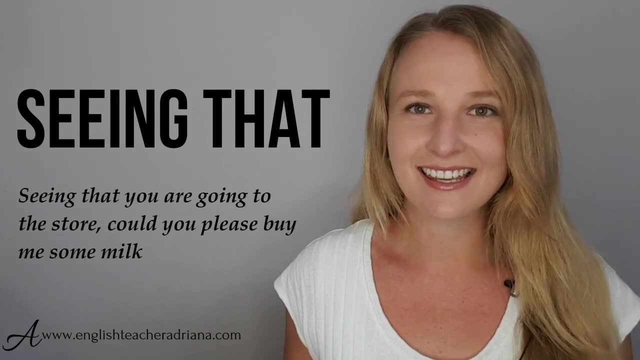 you're going to the store, could you please buy me some milk? This is a great phrase to be using in everyday conversations, instead of because- Careful pronunciation, seeing that, seeing that. But if you need to be more formal, more formal about your relationship in a lookalike setting. 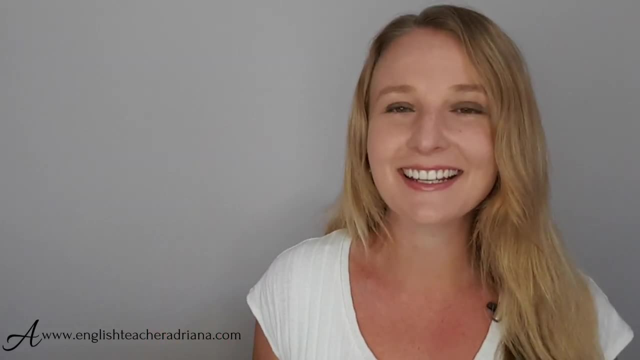 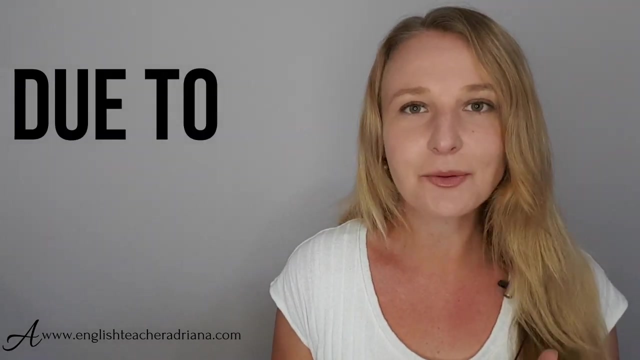 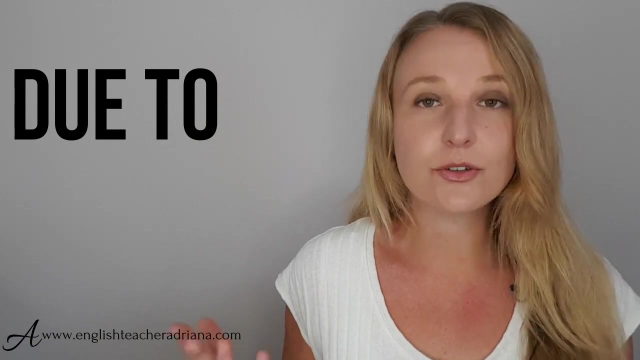 formal than because of a great phrase to be using in this setting is a phrase due to: This is a great phrase to be using in written form in essays and email correspondence at work, to just not overuse because of: If you need to spice it up, use this phrase. I use it a lot and I recommend that you. 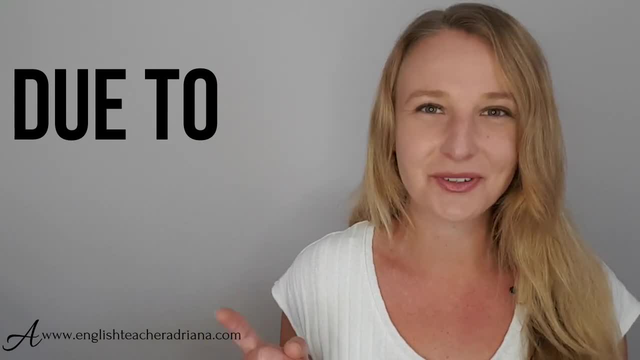 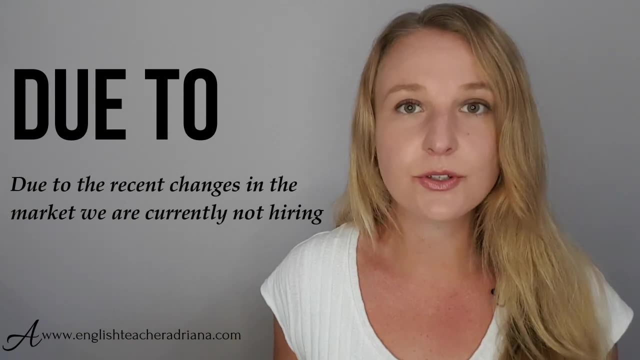 start spicing up your writing, at least by using this phrase. For example, due to the recent changes in the market, we are currently not hiring, So notice here how we're using due to to specifically explain why something will or won't happen Here in this situation, we're talking about the fact. 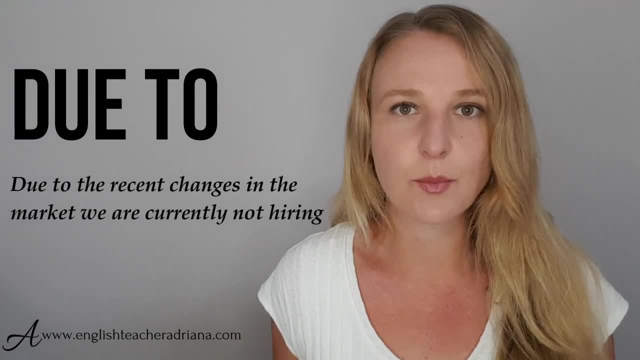 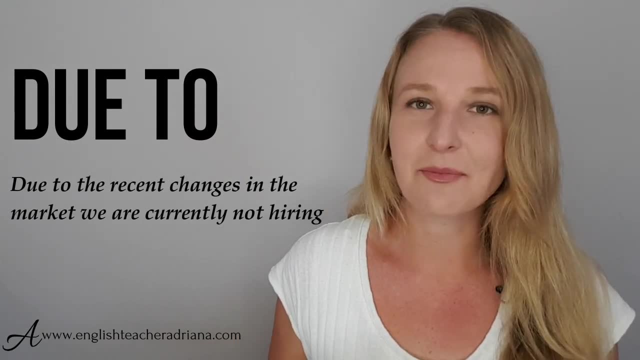 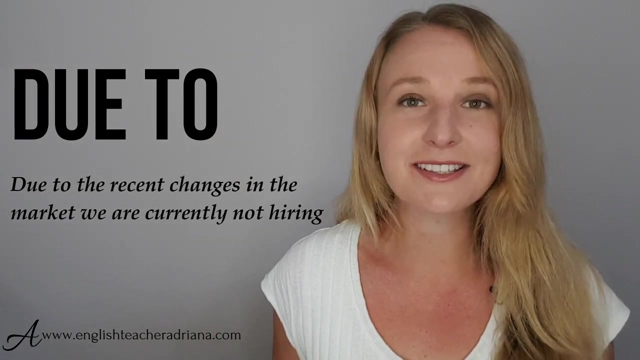 that we won't be hiring, but we could also change a sentence up. For example: due to the recent market changes, we will be hiring. So here, if you would like to explain why something will or won't happen and explain this action, it's a great phrase to be using instead of because of to spice up your 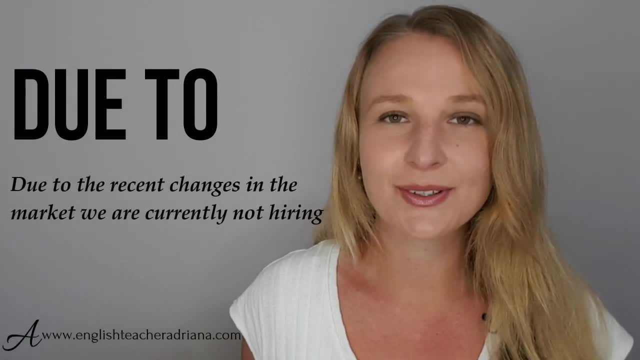 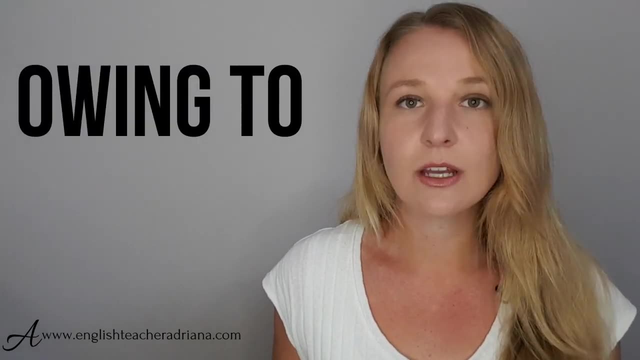 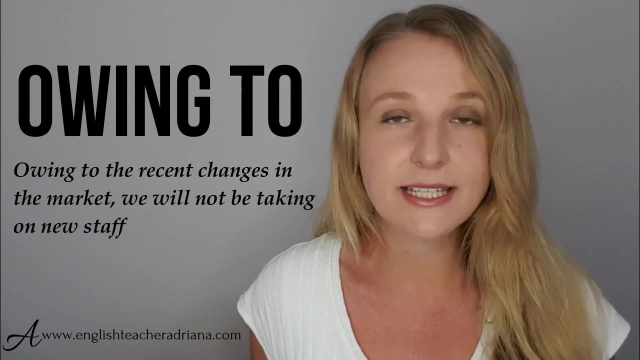 English Careful pronunciation: due to, due to. Now a more formal phrase. the due to is a phrase owing to, owing to. Again, this is a synonym of the phrase because of, For example, owing to the recent changes in the market, we will not be taking on new staff. So here again we're. 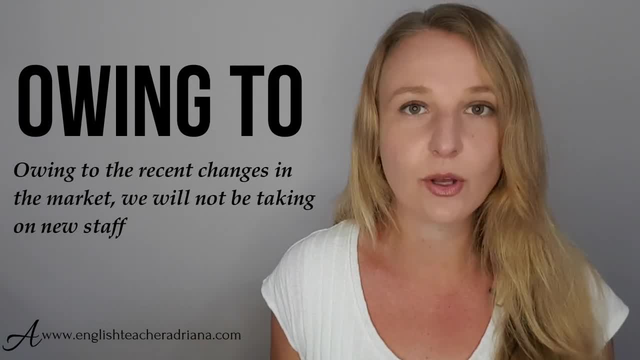 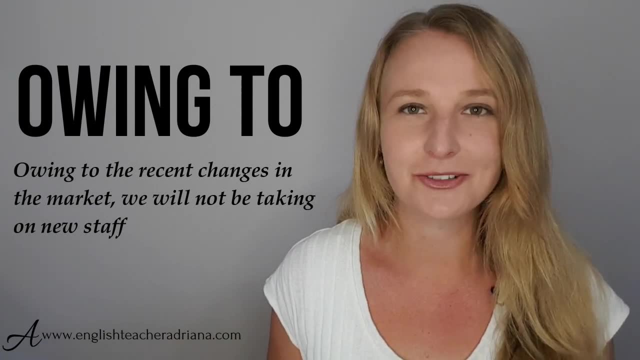 using owing to and stating what has happened and the result that has occurred. after this, It could happen or it couldn't happen. Same meaning as due to and because of. This is a great phrase to be using in essays, in emails, in reports, especially for preparing for. 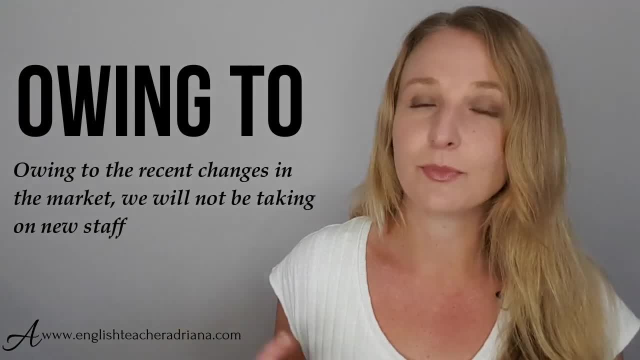 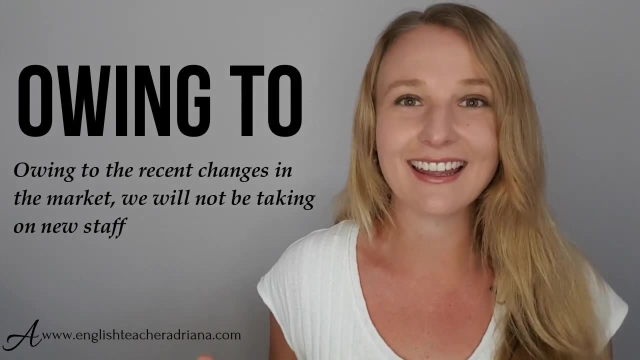 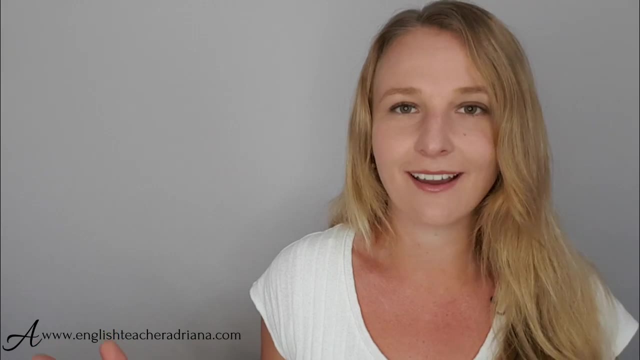 efficiency exams Spice it up a little bit. Owing to is very professional. You can use it in some presentations. It is very formal. If you feel comfortable using it, go ahead and use it. Careful pronunciation: owing to, owing to, Now, if you feel very poetic, a really, really formal way of expressing 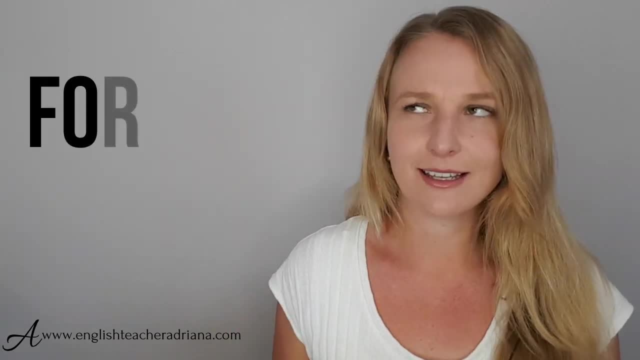 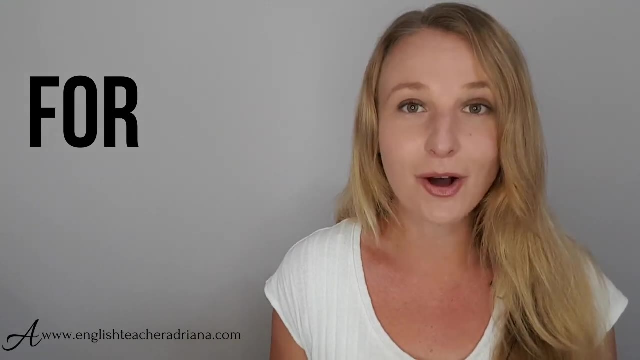 because is simply by using the word for. Now, guys, it'd be a little bit strange if you use for. in everyday conversations I never use this, but when I do say it in poems, in songs, in literature, I know that it means because, and you should also know that this. 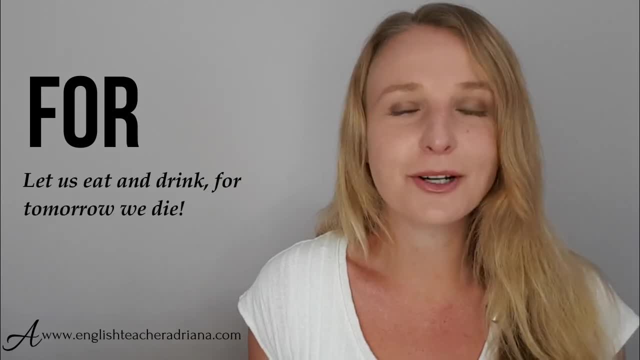 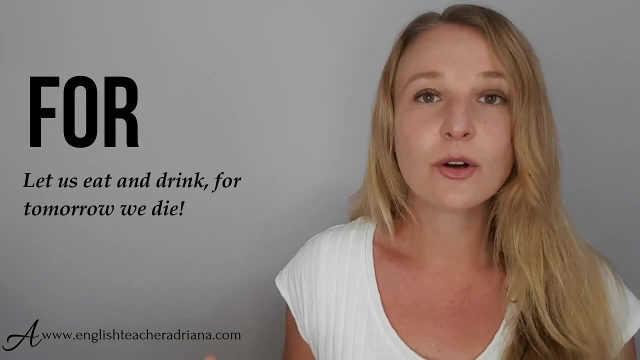 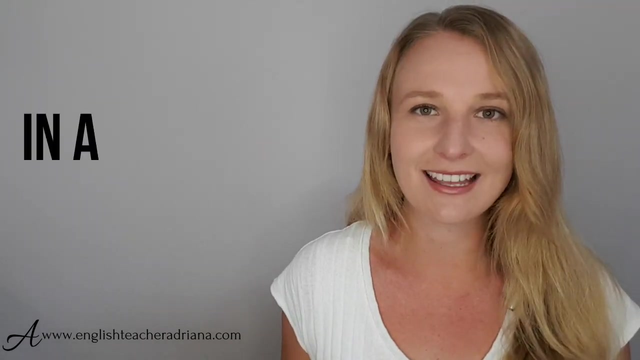 means this, For example: let us eat and drink for tomorrow we die. So this is a really nice poetic way to express because in English, Careful pronunciation for for Now. another really, really formal way of expressing because is by using in as much as, in as much as Guys. this is: 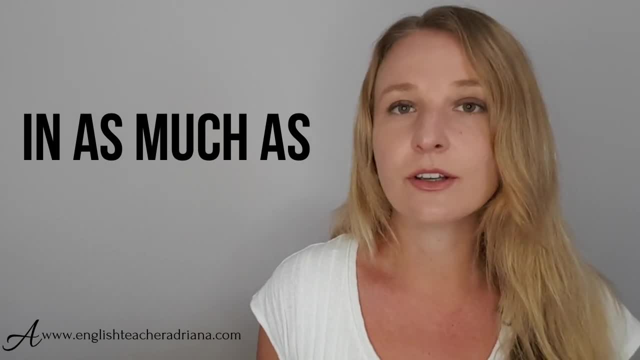 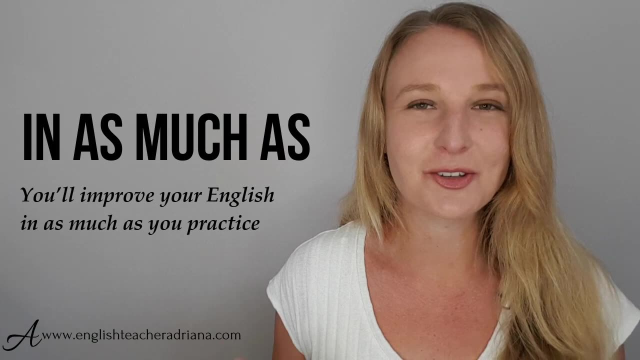 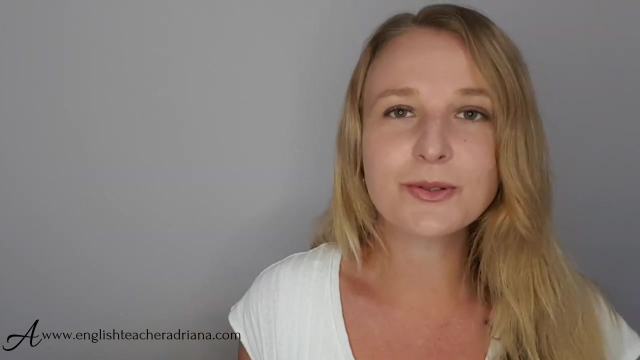 in literature, in reports that you're reading. it's great to know and if you feel comfortable using it, go ahead and use it. For example, you'll improve your English in as much as you practice Careful pronunciation, in as much as in as much as Another really formal, also very proper phrase is a phrase. 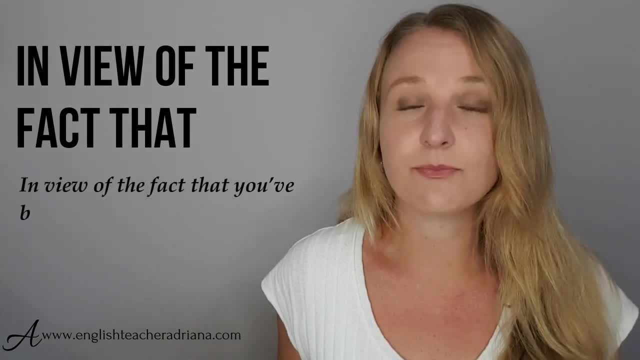 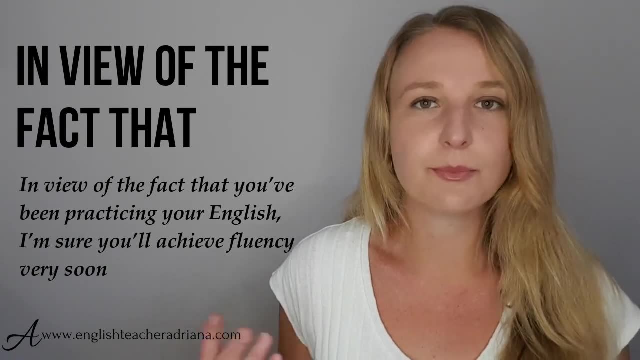 in view of the fact that, For example, in view of the fact that you've been practicing your English, I'm sure you'll achieve fluency very soon. So here, guys, this is a really, really formal, very proper way of expressing, because I don't use this ever. Some English speakers do, If you feel. 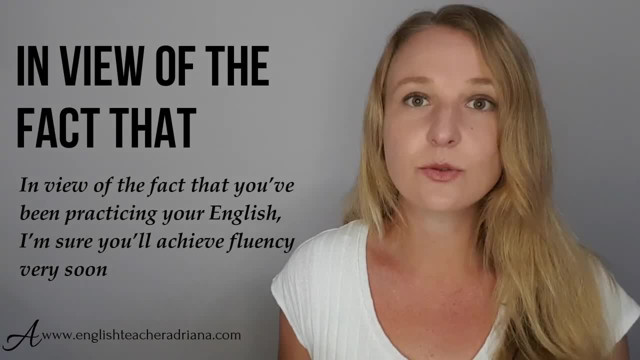 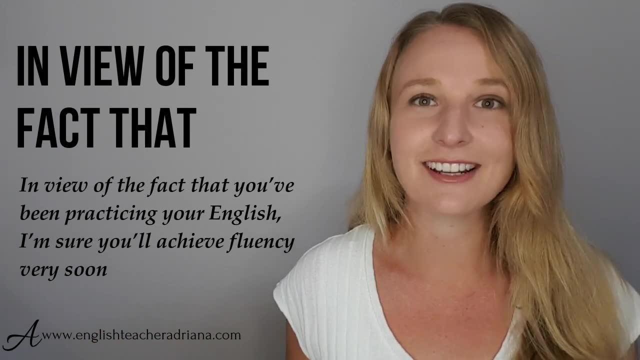 comfortable using this phrase. go ahead and use it, but it is good to know, as you may come across this in literature, in books, and maybe see it while you're at school. but it is a good alternative to keep in mind, to improve your vocabulary. Careful pronunciation, in view of the fact that, In view 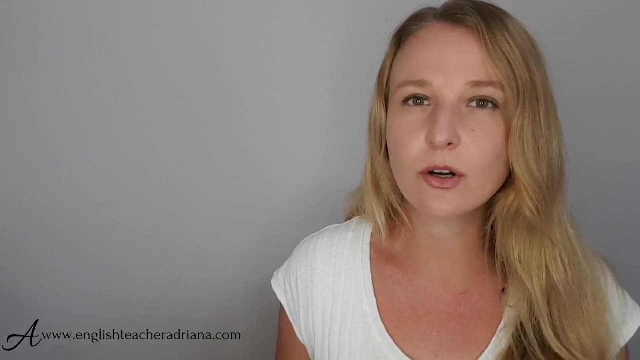 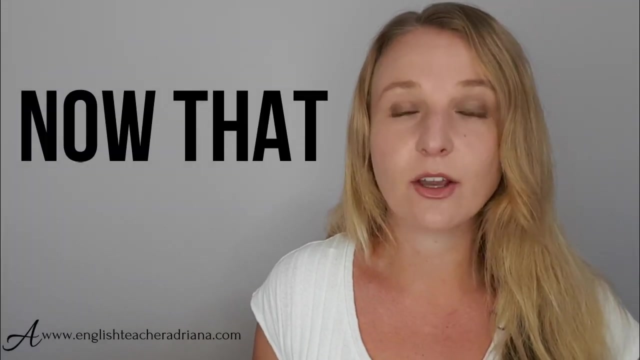 of the fact that Now, a really informal phrase you could use instead of because to express cause and effect- is a phrase Now that, Now that This is really great to be using in everyday conversations with people that you know really well and have great relationships with, For example, now that you've arrived, let's 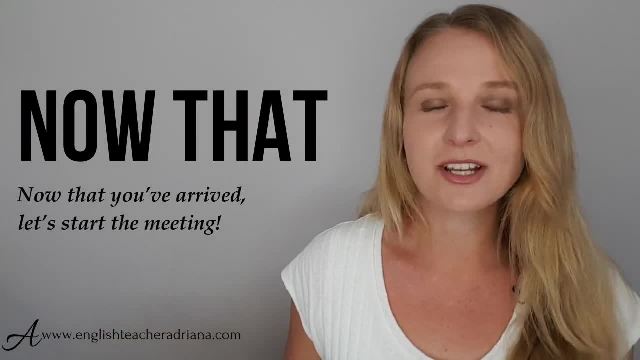 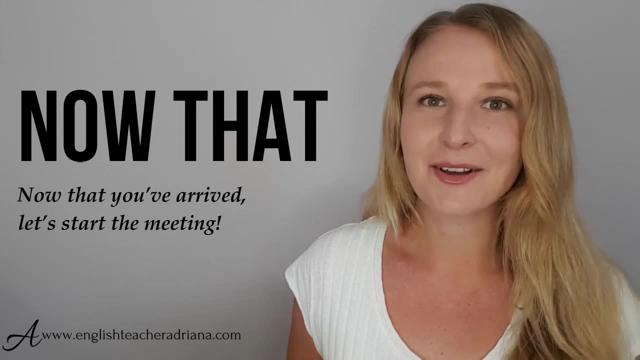 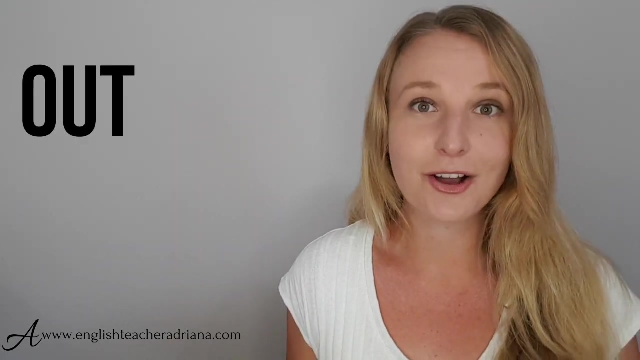 start the meeting. So here you could say: because that you've arrived, or now that you've arrived, let's start the meeting. Careful pronunciation: now that, Now, that Now, if you need to use because for explanations of emotions or feelings, then you could use a phrase out of Out of For. 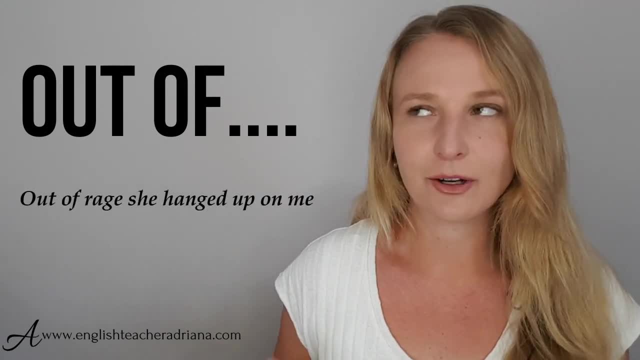 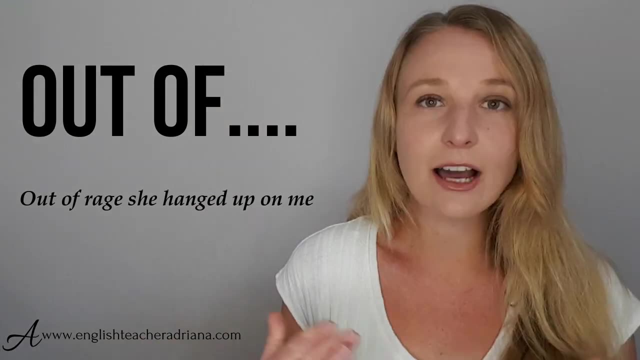 example, Out of rage, she hanged up on me. So, for example, I called Mary and just out of rage, she just hanged up. Yeah, I could say because she was angry or because she felt angry. Out of rage is very advanced. It sounds very professional and it's a great phrase to be using if you're writing stories. 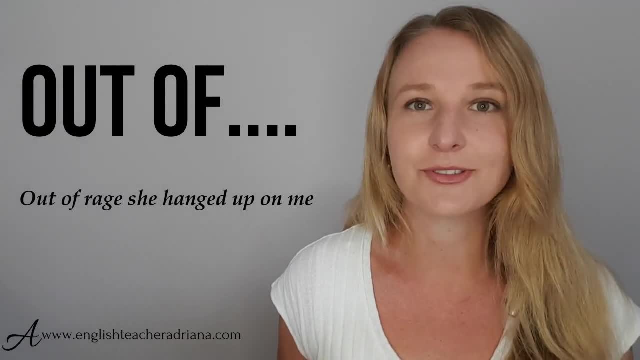 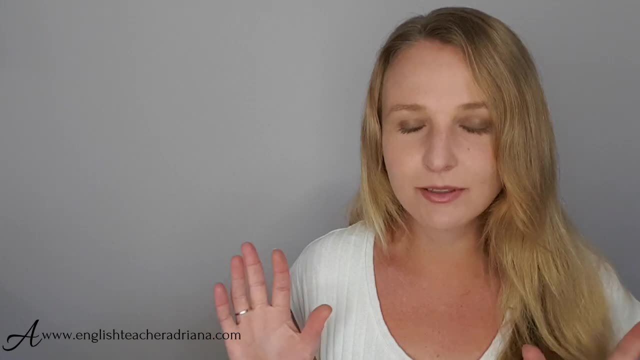 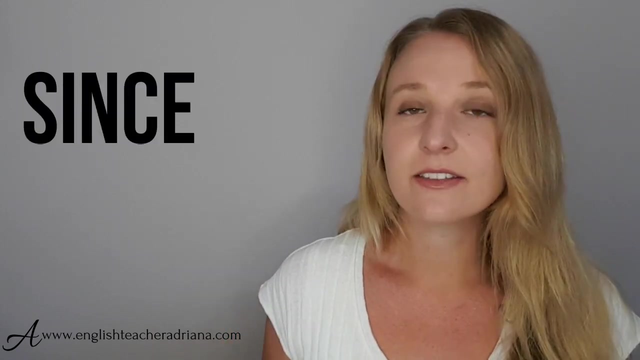 writing essays in formal situations, you may find yourself in Careful pronunciation out of Out of Now. the next word you could use instead of because is probably really confusing for you guys, but I'm going to touch base on this, And that word is since, Since This is really informal. For example, I 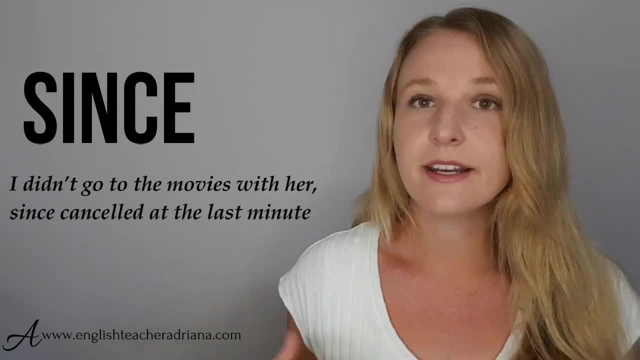 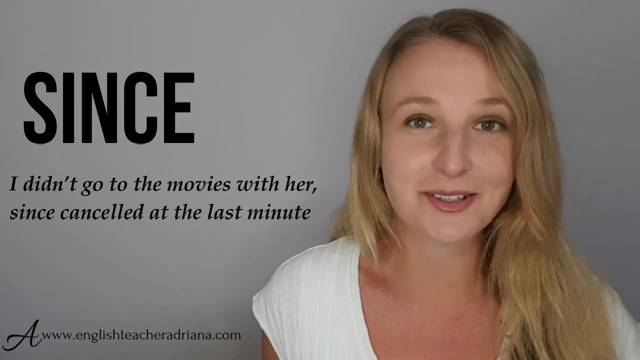 didn't go to the movie with her since she cancelled at the last minute. Now here, since is being used instead of because. So a lot of English speakers use this in everyday conversations. I use this a lot And if we simply use it instead of because as a synonym, It is very informal, I don't suggest 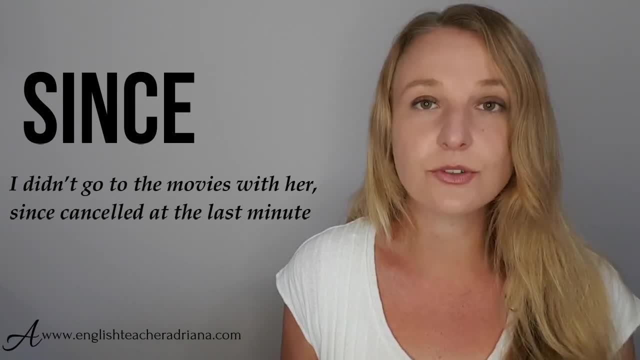 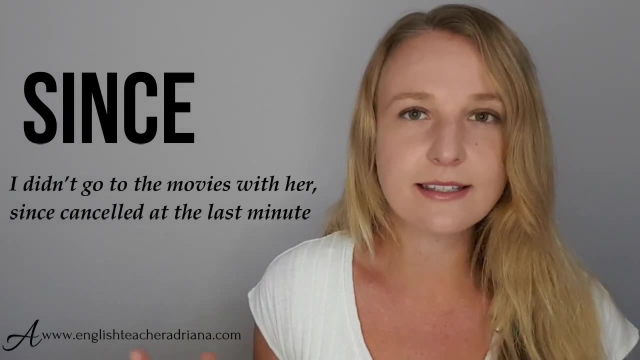 that you use this in written correspondence, in emails, But it is great to know that this means because, in certain situations. So I'm going to touch base on this, And that word is since, Since. But please pay attention when you're reading something, When you're listening to people Pay. 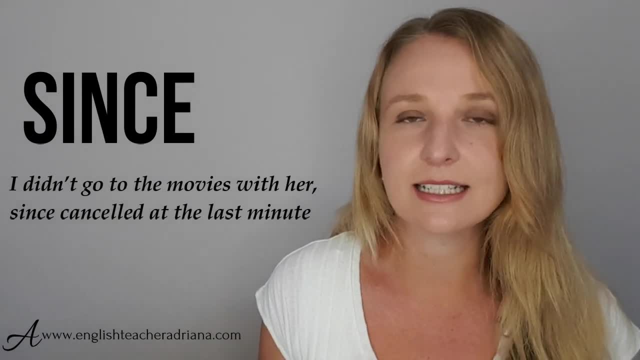 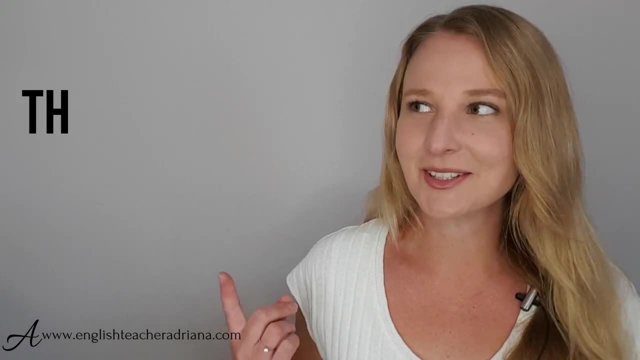 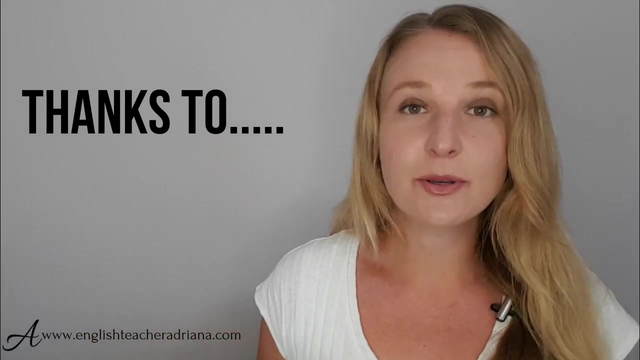 attention to the context and if there is some sort of cause and effect in that situation. Careful pronunciation, Since, Since, Also the phrase thanks to, Thanks to Can mean because in some situations- Now, if you're confused about this, stress less, Because thanks to can have a positive. 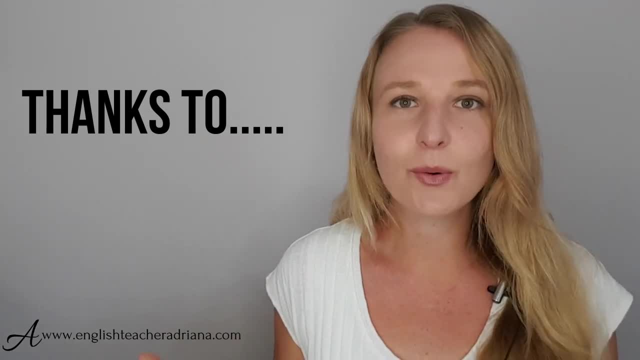 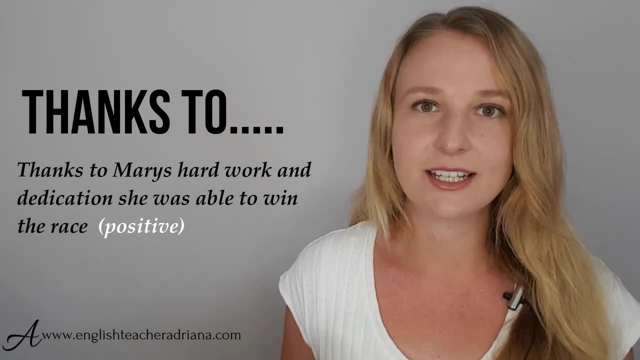 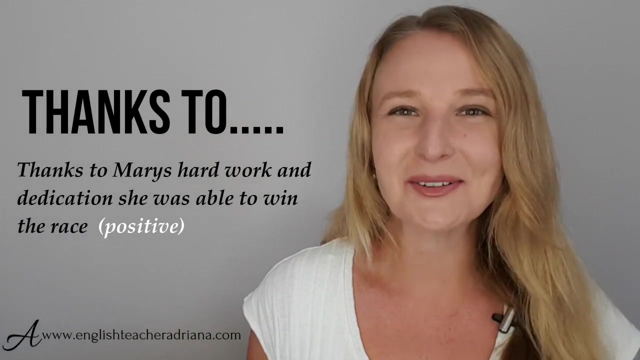 connotation and also a negative connotation. For example, Thanks to Mary's husband. Thanks to, Mary's husband slept in the car. Because of her hard work and dedication she was able to win the race. So here, Thanks to is being used in a positive connotation. So because of her hard work and her 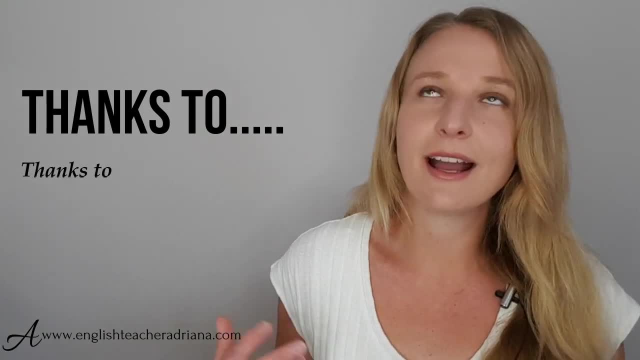 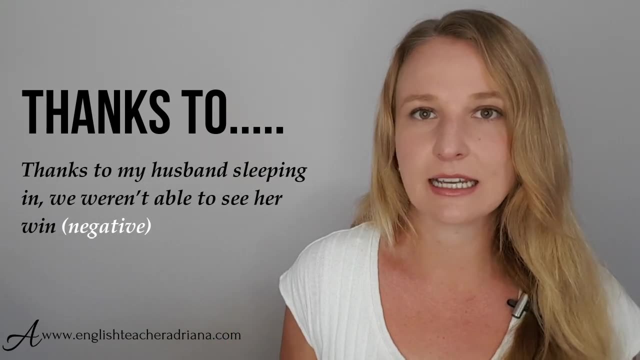 preparation, she won the race. But we can also use it in a negative connotation. For example, Thanks to my husband's sleeping in, We weren't able to see her win. So here, Thanks to is being used in a negative connotation, Because we really wanted to see Mary's race, But my husband slept in And here. 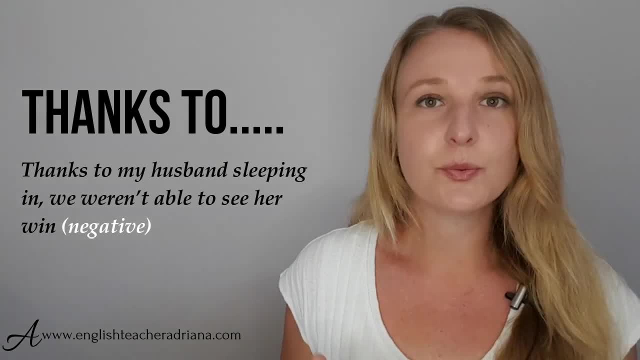 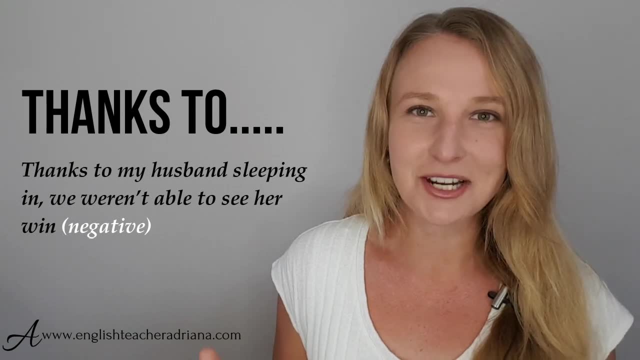 used in a negative way to express because of. You will hear this used a lot in TV shows, in movies, in everyday conversations. Be aware if there's a positive or a negative connotation. It is a great phrase to be incorporating with speaking in English and also pay attention to the intonation. 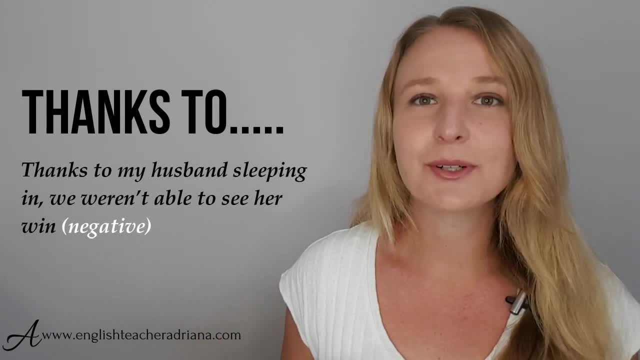 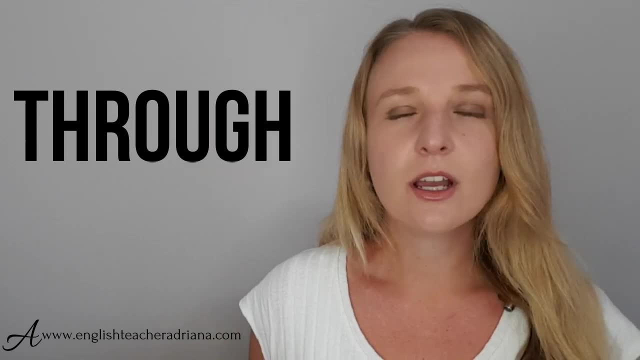 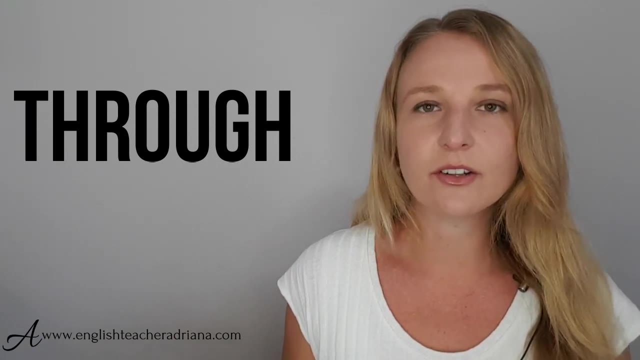 that you use, depending on the connotation, Careful pronunciation: Thanks to, Thanks to You could also use the word through Through To be very polite and very proper. this is really good to be using in written form when we're talking, when reporting on certain